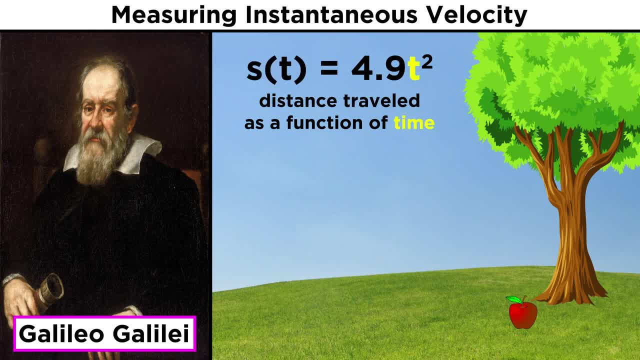 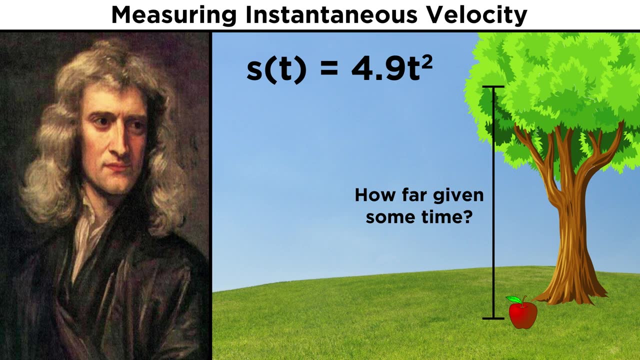 object represented by s of t would be equal to four point nine t squared with t in seconds, giving a distance in meters. So Newton could easily use this law to calculate how far something would fall over a given interval of time. But this was not the problem at hand. 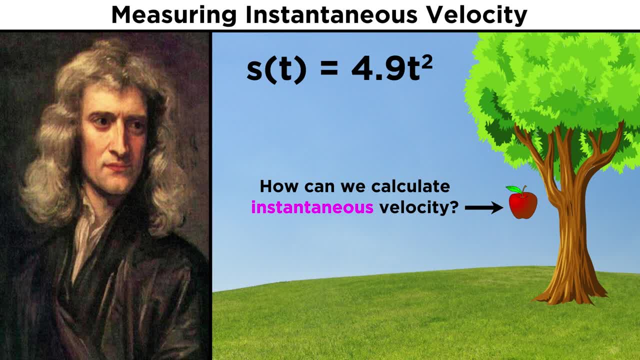 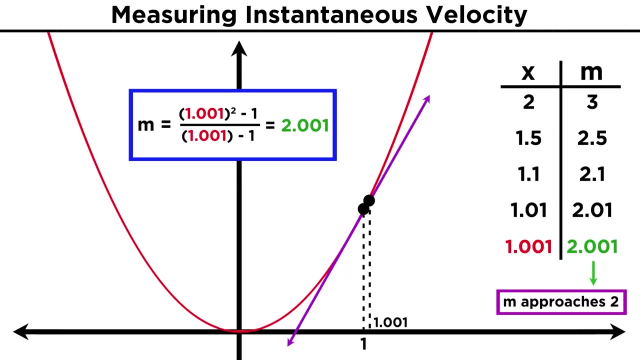 Newton wanted to know something not about an interval of time, but rather about an instant in time, like perhaps the velocity of the apple precisely five seconds after letting it fall. Well, just like we did in the previous tutorial with the secant and tangent lines, let's 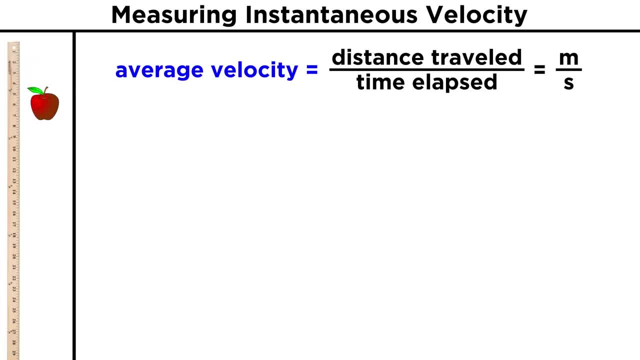 make an approximation. We can calculate average velocity by taking some distance traveled. Let's make an approximation. Let's take some distance traveled and dividing by the time elapsed, as that will be meters traveled over seconds traveling or meters per second, And using Galileo's equation, we can express distance traveled as the difference between: 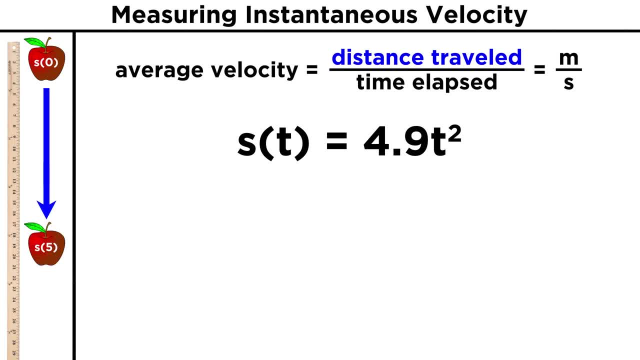 two points in this function. Say, we use the distance traveled after five seconds, or s of five, and the distance traveled after six seconds or s of six. If we subtract the former from the latter, we are going to get the distance traveled. 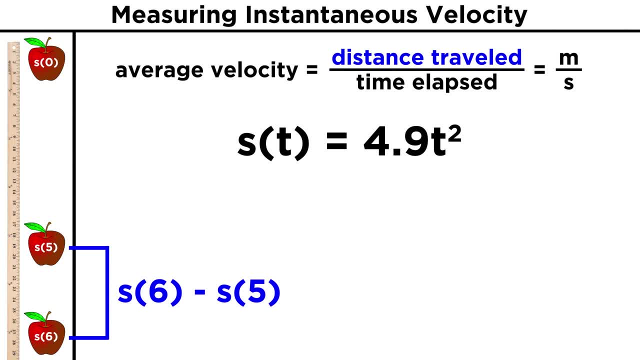 after five seconds or s of six. If we subtract the latter, we are necessarily describing the distance traveled during the period from five to six seconds. after being dropped, That will also mean that the time elapsed is one second. So we just evaluate the functions for these two inputs and subtract. 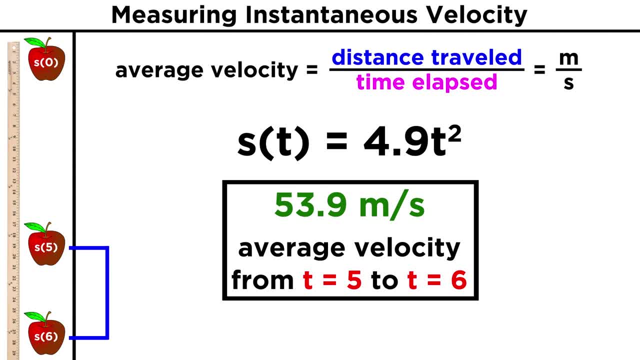 Divide by one second and we get fifty-three point nine meters per second. So that is the average speed of the apple during that one second interval. But remember, we don't want an average speed, We want the precise speed at a precise instant. 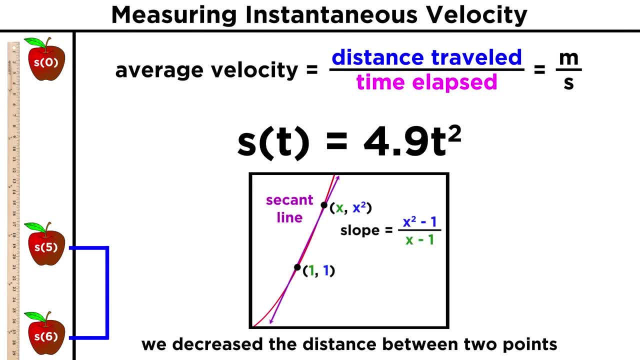 So what do we do? Well, just like the way we nudged the second point in the line closer to the first until we got the tangent line for the curve, let's nudge the end of this time interval closer and closer to five seconds.